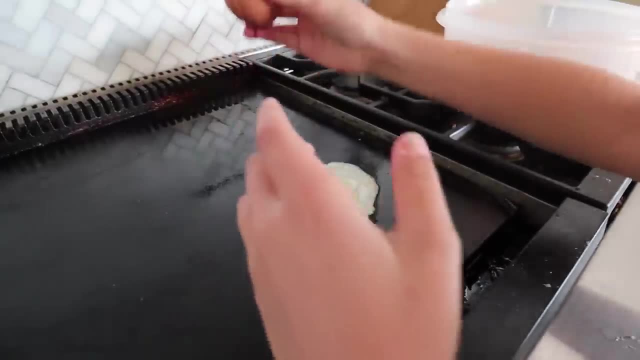 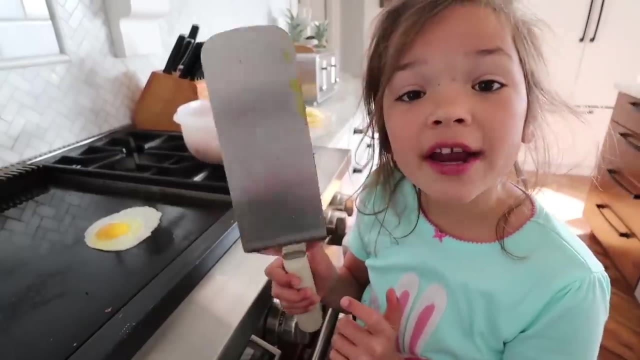 The key to the best sunny-side up eggs is to spray the griddle in the TV. Gotta spray the griddle in the TV, so it's legal eggs- is to make them a little bit runny. So when you flip them try not to break the yolk. 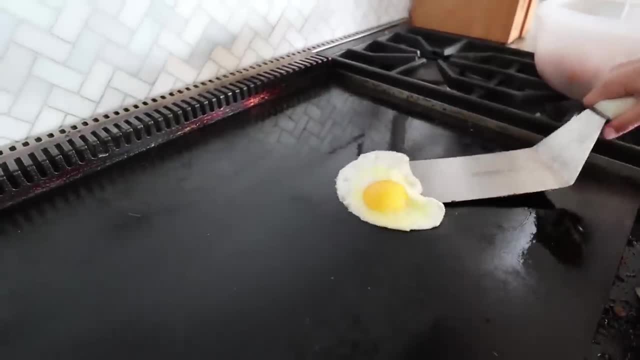 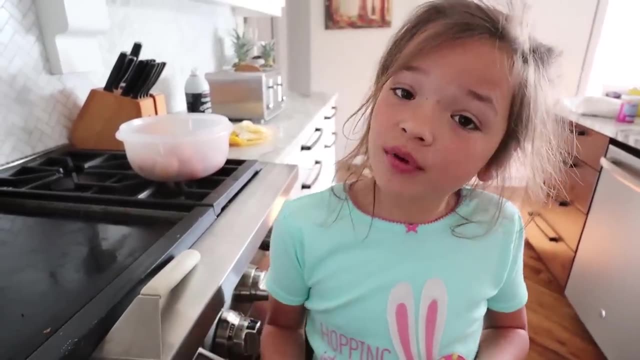 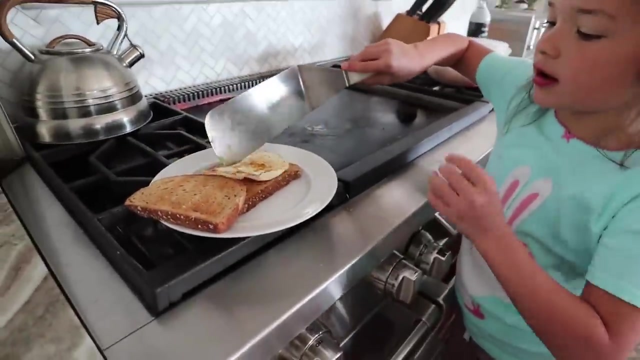 or else it will not be runny. See, while the egg is cooking, we pop our bread into the toaster And then we just wait, Flip it and put it on, and then I put this one on so that it's an egg sandwich. 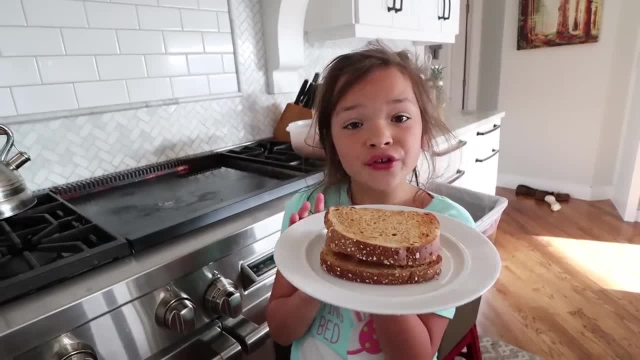 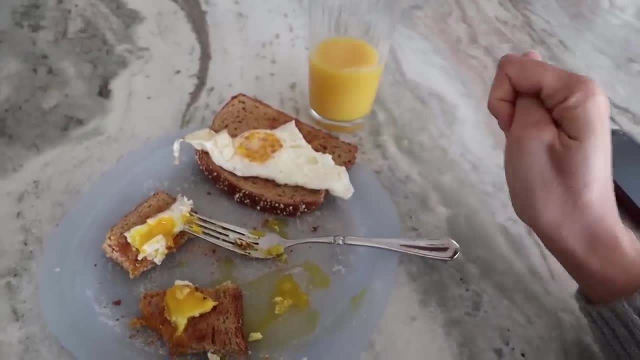 Super easy and less than 10 minutes to cook. Serve it with fruit or orange juice and we're ready for breakfast. I am halfway done with my meal: Orange juice, eggs on toast- That's good- greens and protein and fruit juice. So I think that's a good start for our breakfast. 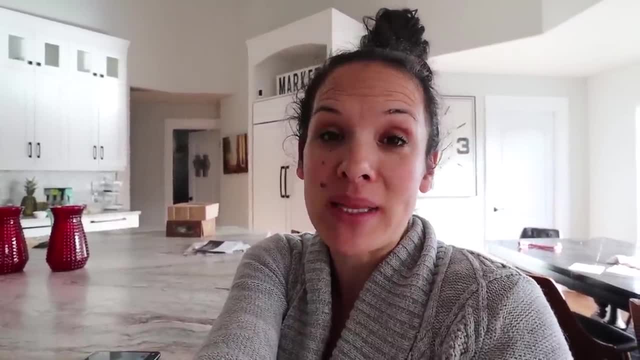 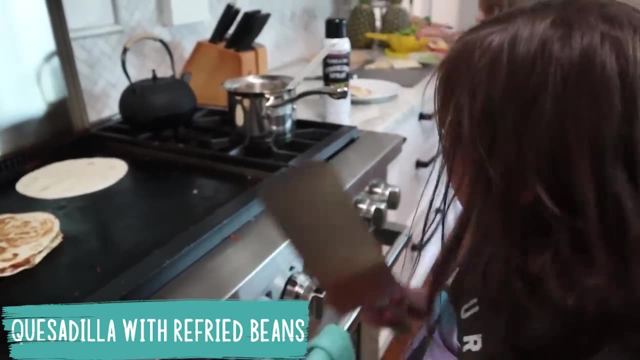 We also like to add in fruit, and I think that completes our meal. Way to go, Evie. On to the next meal. The super easy dinner is quesadillas with refried beans. So we didn't have a can of refried beans. 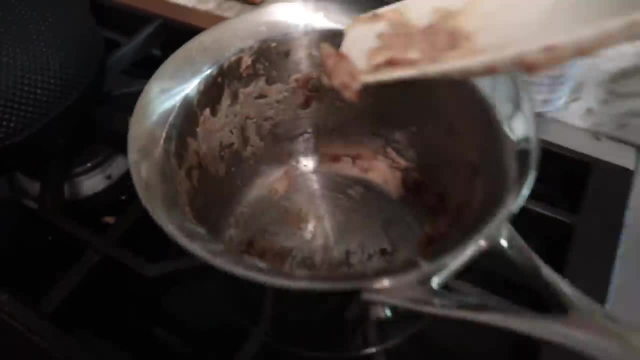 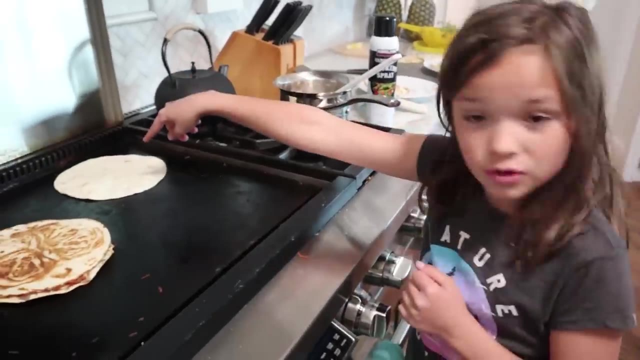 but we did have a can of quesadillas with refried beans, So we got pinto beans and cooked it our own Best to do it on the plate before the griddle, And you gotta spread it around. Then you put one tortilla on the griddle. 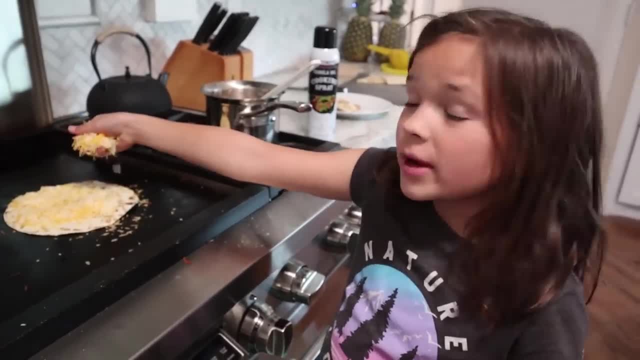 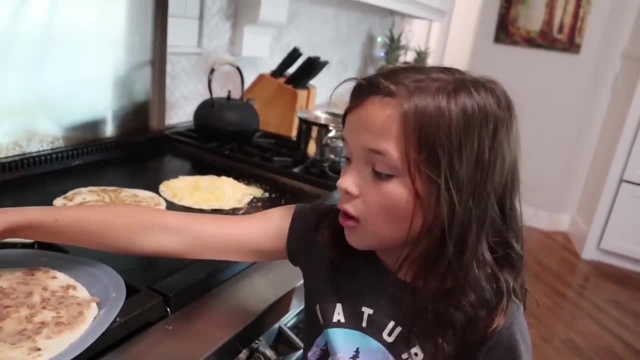 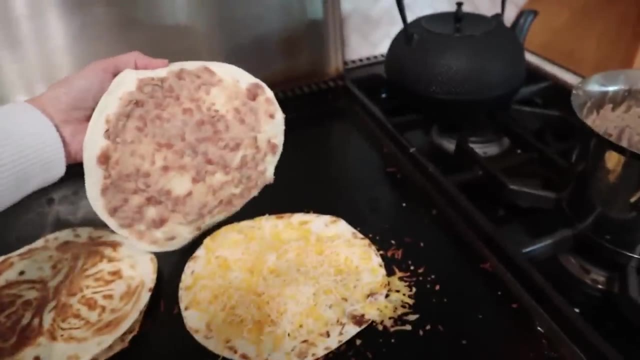 Then you add cheese onto it, Then you put some more cheese on it and always make sure you have adult or teen superfood. Add your quesadilla with pinto beans on it. This part might need more adult supervision, so you're gonna add it like a sandwich. 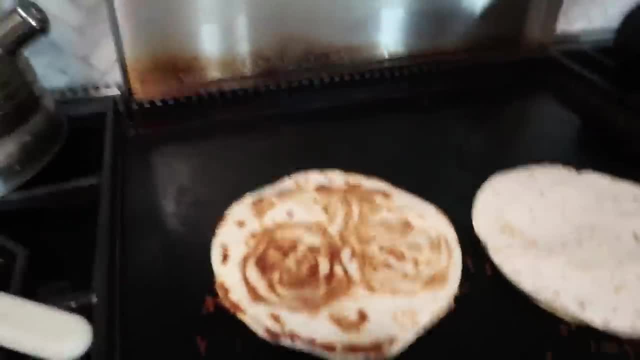 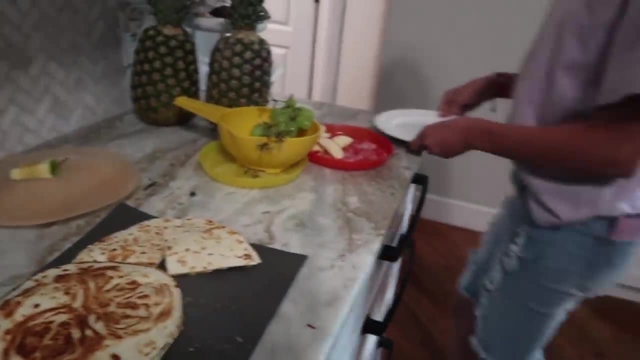 Let it cook for a little bit and then you're gonna flip it over And then it's done And we're gonna cut them up And Evie. what are we serving it with dinner tonight? We're serving it with grapes and apples. 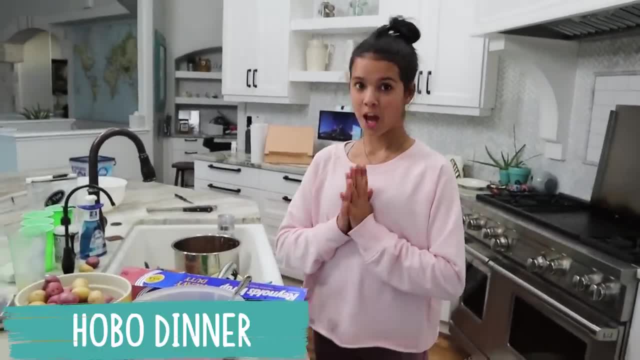 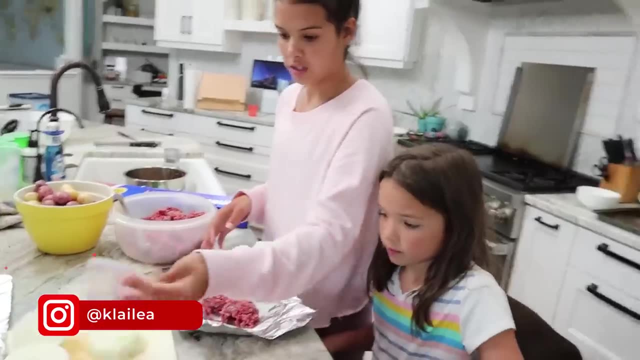 We haven't had any apples, All right. another easy meal kids can cook are what Hobo dinners? So we have got the meat. You just scoop some meat into your tinfoil. Okay, you want some onions? No, No onions. 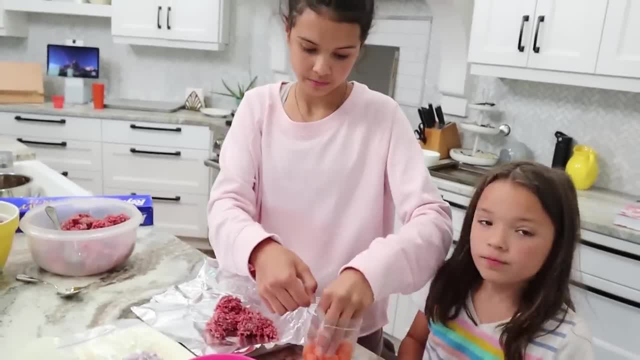 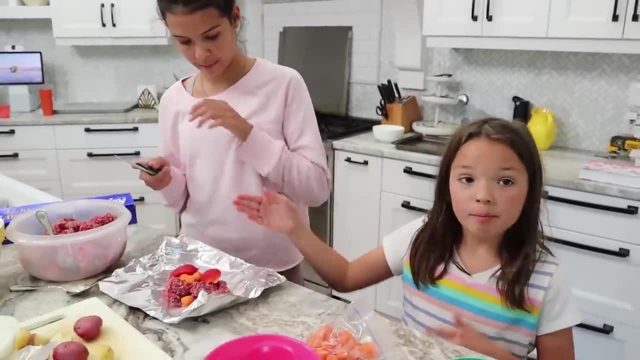 You want some carrots? Yes, Just a little bit. Just a little bit. Two, Remember: onions and carrots is what flavors the meat. Two: All right, we're adding vegetables to it. What are you adding, Evie? I added these bell peppers. 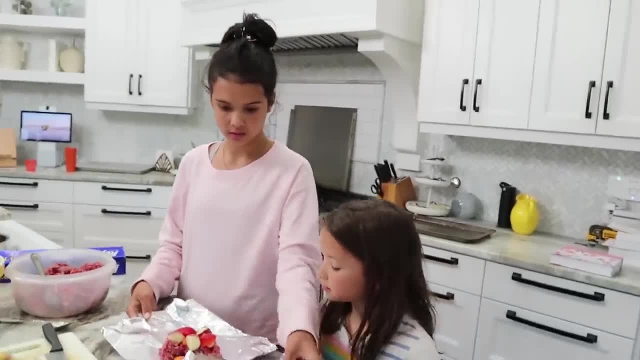 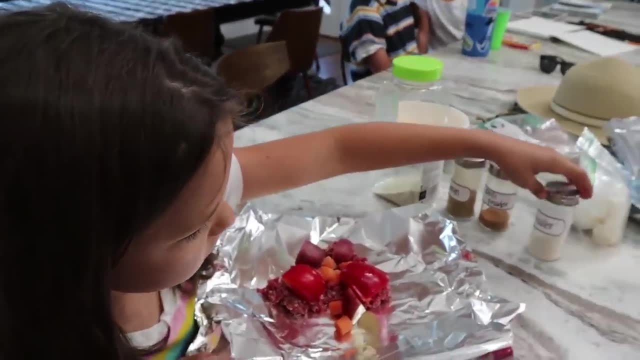 And now Do you want some potatoes? Yes, Now the next step is really easy. What do we do? Spices, You can add your spices. You can add some chili powder if you want it to be like tacos, or you can add like steak seasoning. 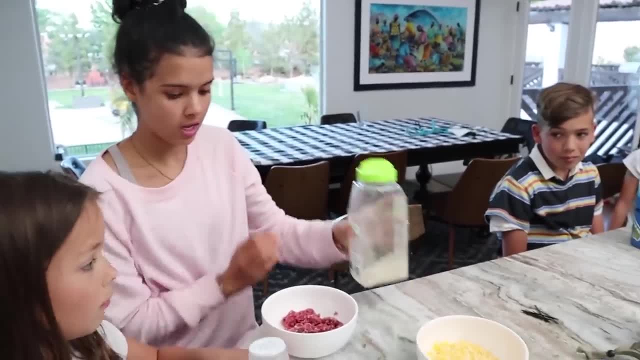 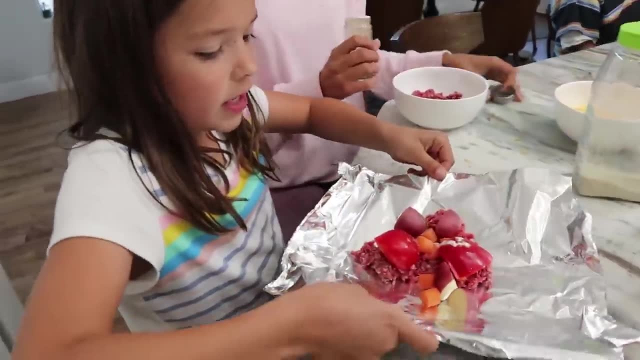 What does onion powder taste like Onions? Hey, what are you doing? I just decided I'm gonna try putting the meat in a bowl and then I'm gonna add my spices. Evie, are you done with your spices? Yes, 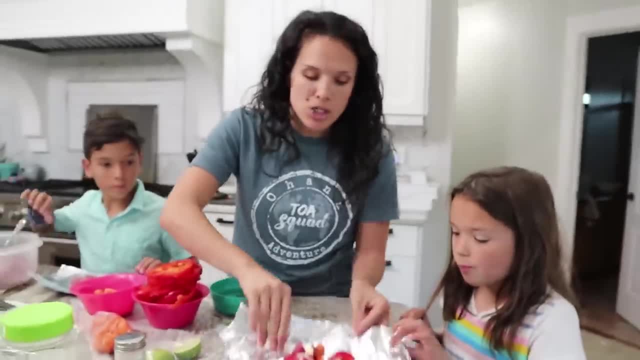 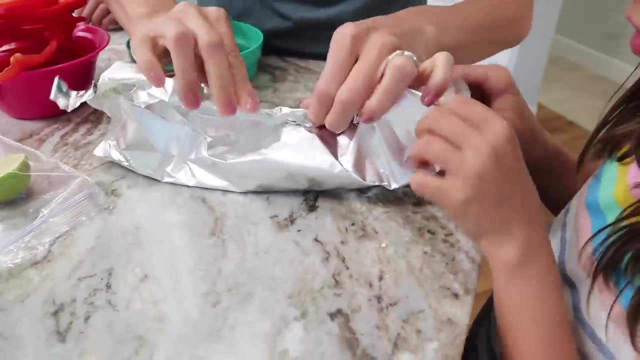 Okay, so we're gonna wrap it really good. All right, this is how you wrap, guys, Everyone pay attention. You're just gonna wrap it up. You can do a kind of like a burrito style, where you fold this over. 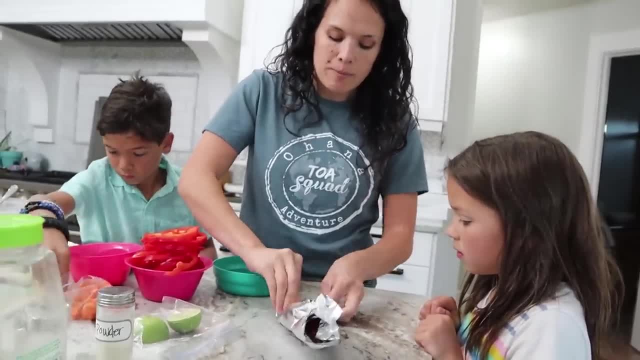 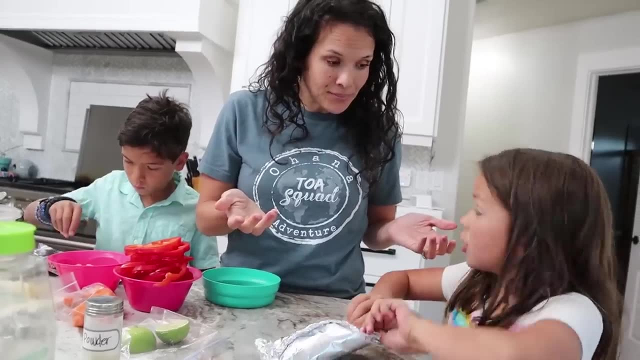 And then you're wrapping up the ends. You roll it up like this: Can you roll up that end, That end, that end? Okay, and now what do we do? Cook it? Yep, we cook it. We're gonna cook it in a fire. 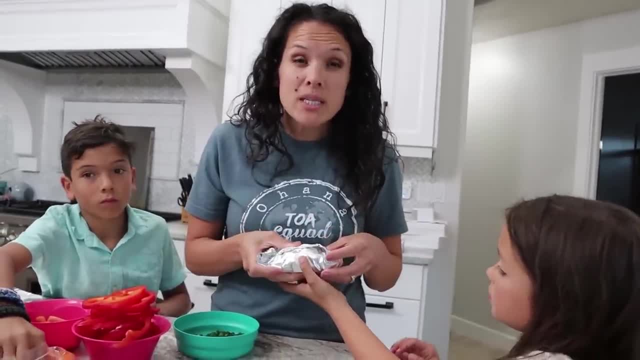 So this is a hobo dinner. We prepare this at home and a lot of Boy Scouts take them with them when they go places, Or Girl Scouts, Or Girl Scouts. But we have a fire pit outside, so we're gonna cook our dinners outside. 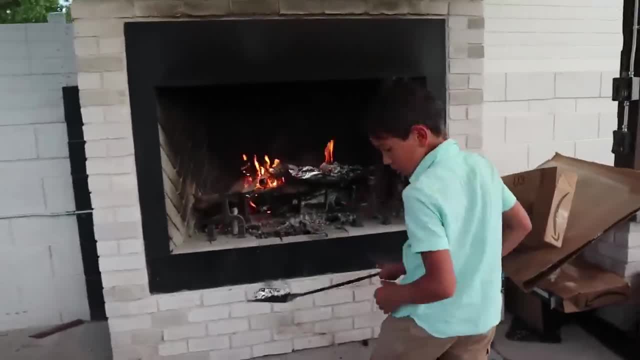 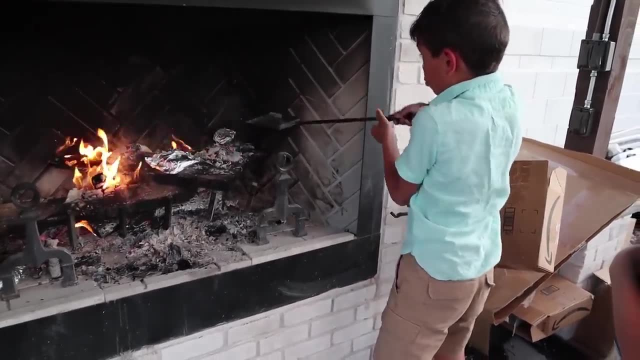 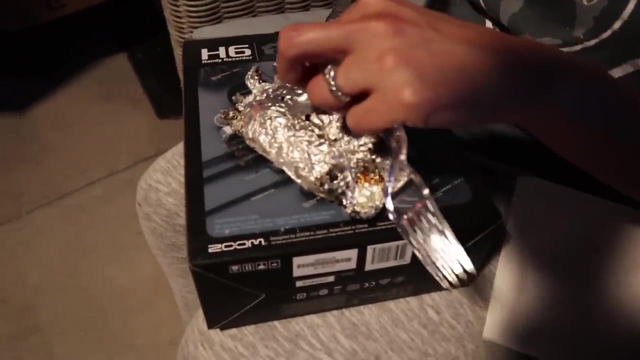 All right. so our next step is putting in the hobo dinners. Wyatt's gonna go and put his in. There you go. Okay, we are opening up our hobo dinners. They've been in the fire. They are very hot. 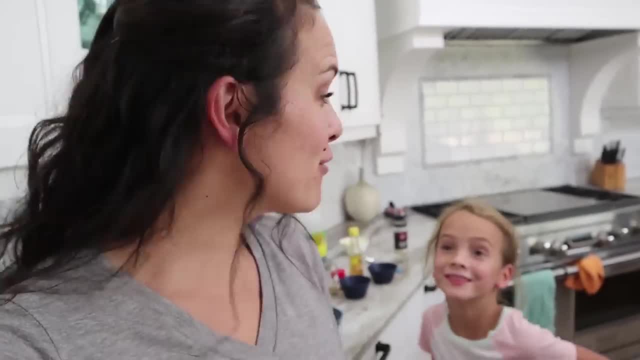 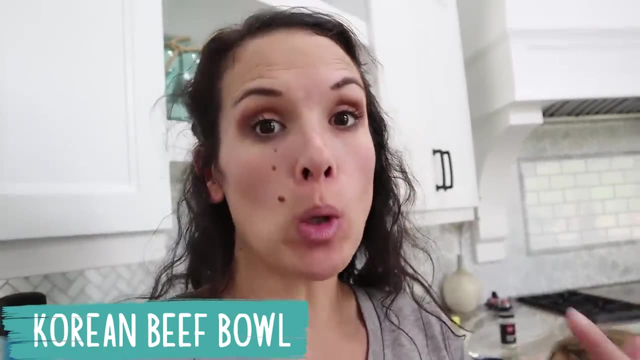 Then we will eat. All right, we have a favorite easy meal that Cora's gonna cook tonight, And what's it called? Korean beef bowl. All right, I love the bowls like teriyaki bowl, chipotle bowls, Hawaiian haystacks. 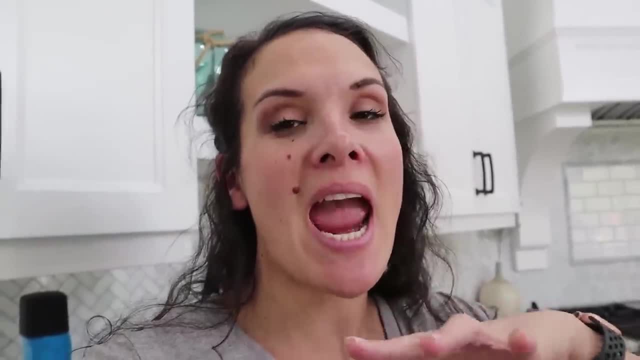 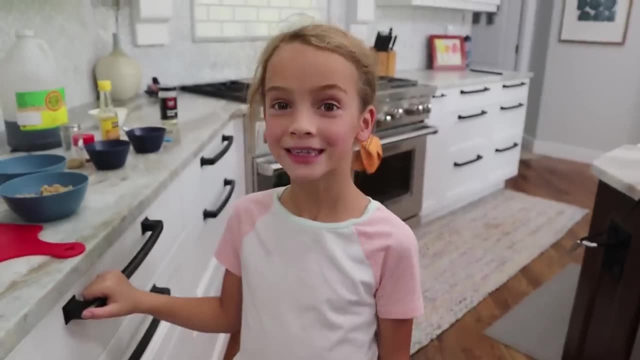 all those sorts of meals because you can shove in a bunch of vegetables and make a big bowl full of vegetables and the meat and the sauce and rice. It's super fun and easy. The kids love these types of meals. First, you need some ingredients. 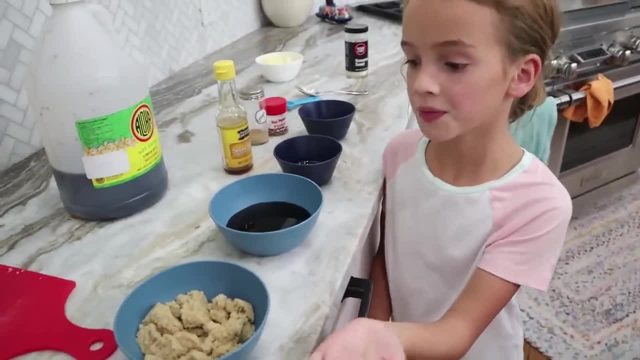 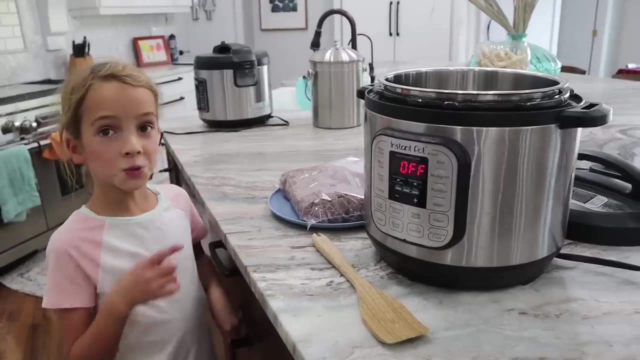 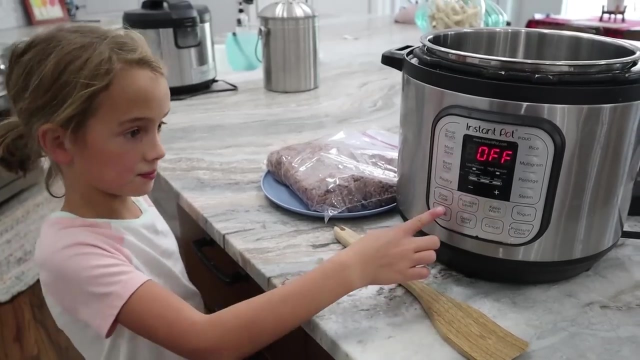 Chopped up garlic, brown sugar, soy sauce, sesame seed oil, ginger, red pepper flakes. First, we are going to cook the meat in the Instant Pot, so we don't use the stove First, let's turn it on. Saute your ground beef with your garlic.